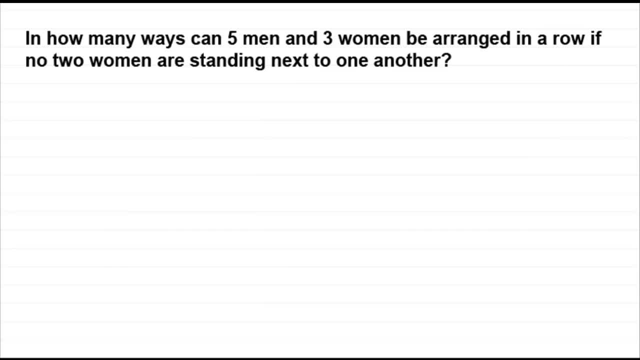 And I'm going to do two examples for you. The last one you might even want to try yourself, based on this one. Now, what we've got here is: in how many ways can five men and three women be arranged in a row if no two women are standing next to one another? And to do 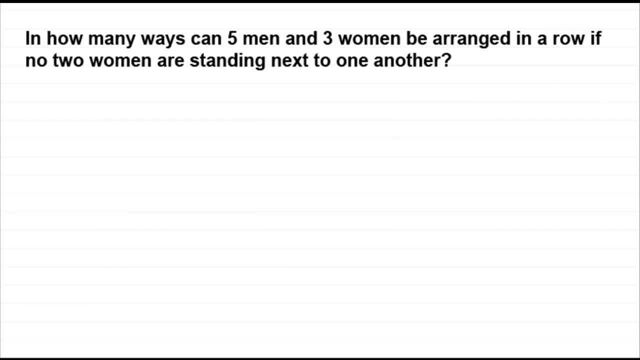 something like this. what I would suggest you do is put down some spaces, And what we're going to do is fill those spaces with, with the five men first of all. Then we're going to look at the three women, Now the five men. what you do is you put them down in such a way that you leave a space between. 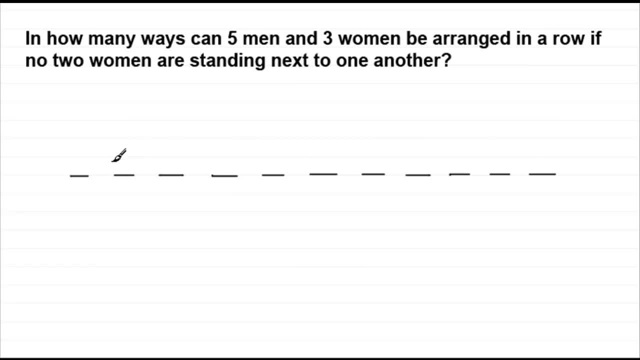 each one of them. So we'll put the first male down in this space here and we'll call it M1.. Then we'll put M2, M3 and so on. okay, until we have put down however many items that are in the question. 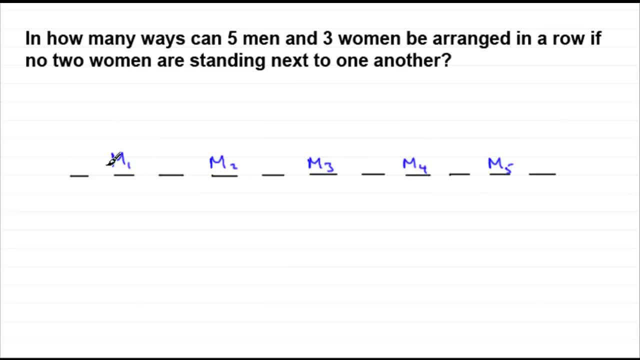 So we've got our five men here, leaving a space in between each one of them. Now, how many ways can those men rearrange themselves amongst themselves? okay, That's the first thing, What we've already seen in the past, that if that were the case, then N items can be rearranged. 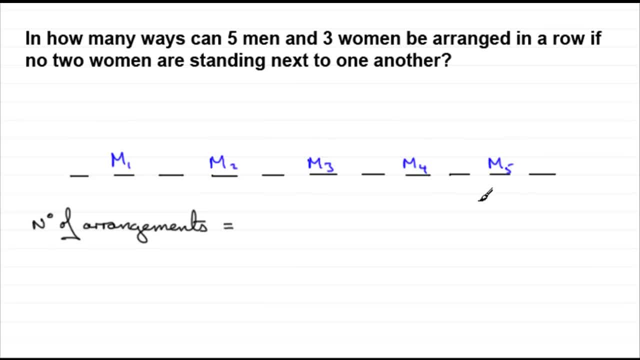 amongst themselves, as long as they're different. N factorial ways. So in this case it's going to be five, Five factorial ways, Five times four times, three times, two times one. Now if we look at the women, okay, let's just put them down here: W1, W2, W3 for the three women. Now, 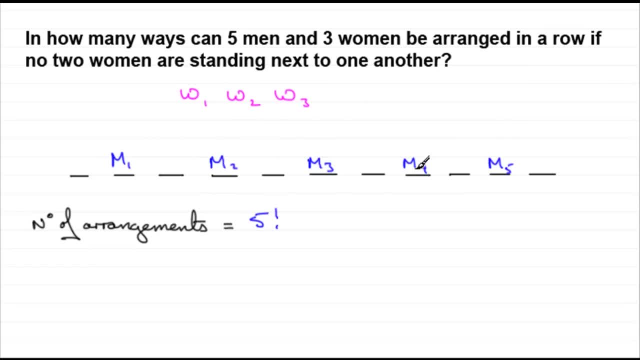 for any time that we have an arrangement of the men, any of these five factorial ways. a woman has a choice of 1,, 2,, 3,, 4,, 5,, 6,, 7,, 8,, 9,, 10,, 11,, 12,, 13,, 14,, 15,, 16,, 17,, 18,, 19,. 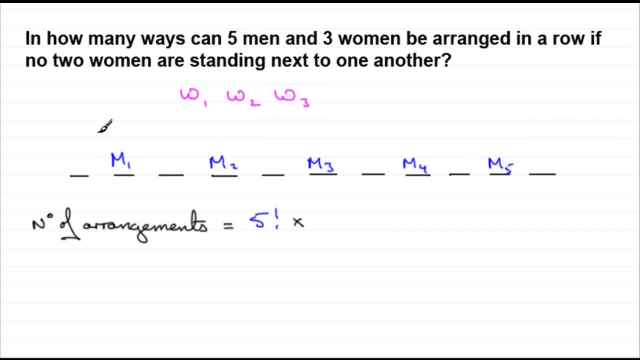 20,, 21,, 22,, 23,, 24,, 25,, 26.. Six places to stand. okay, That's the first woman. So there's going to be six ways for a woman to stand somewhere in one of those spaces. But as soon, 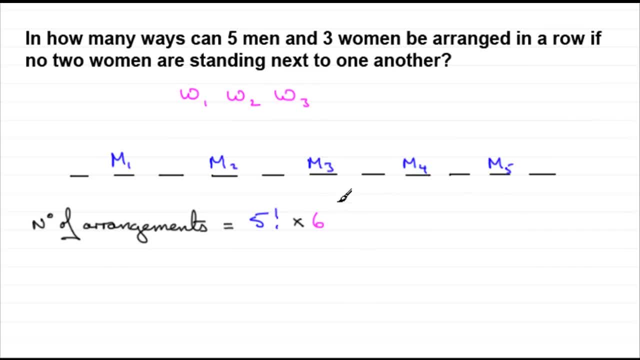 as that woman is in one of those places. the second woman has a choice of just five more spaces, So there's going to be five times there And for any of these places you're these five places. the final woman has only got a choice of four spaces, so it needs times. 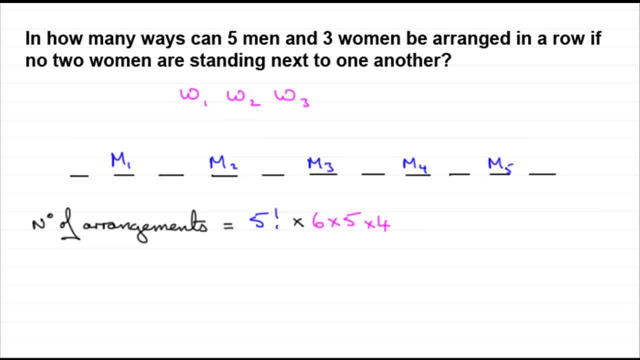 by four. So if you were to work this out, what you would find is that you get 14,400 different arrangements of how these people can stand. Okay now, I did say that this tutorial consists of two examples, and the second example is: 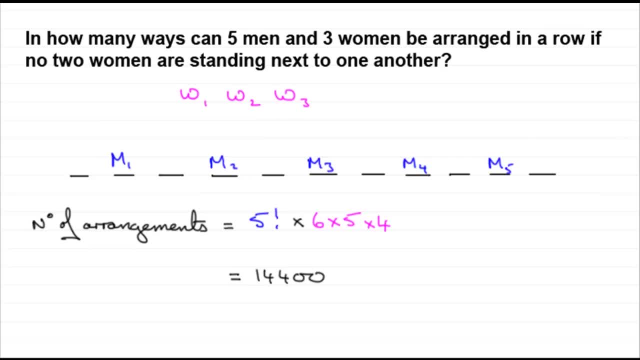 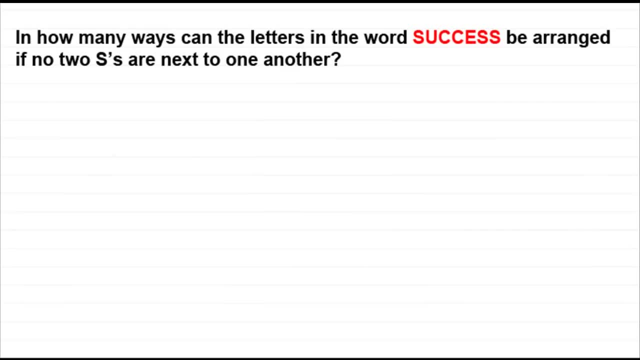 a bit harder than the one that we've just been doing. Now. what we have here is: in how many ways can the letters in the word SUCCESS be arranged if no two S's are next to one another? Now you might like to pause the video and 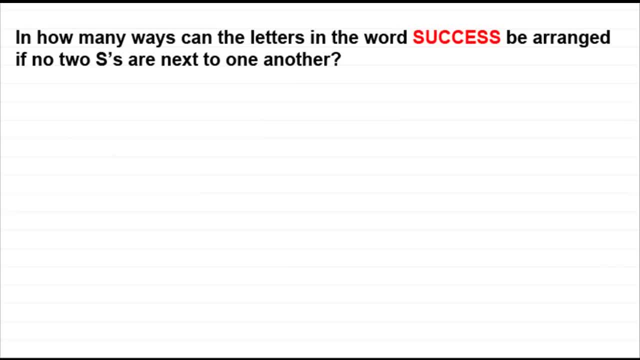 come back when ready and I'll work through the solution for you. Okay, you might like to just check to see whether you're able to do it. Okay, welcome back. if you had a go Now for this one, what I would do is, first of all, 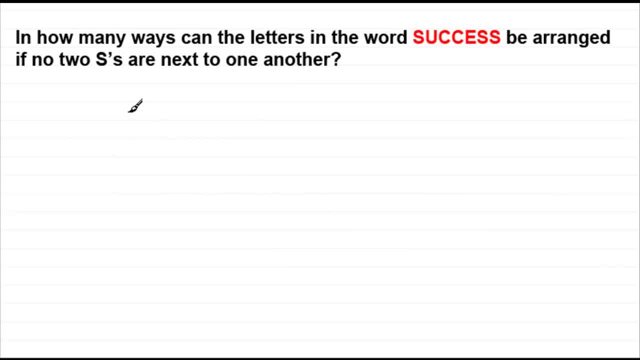 put down the letters U, E, C and C, the ones that aren't the S's. So I'm going to put down the letters U, E, C and C and then the letters S's. So let's just put those down here. We've. 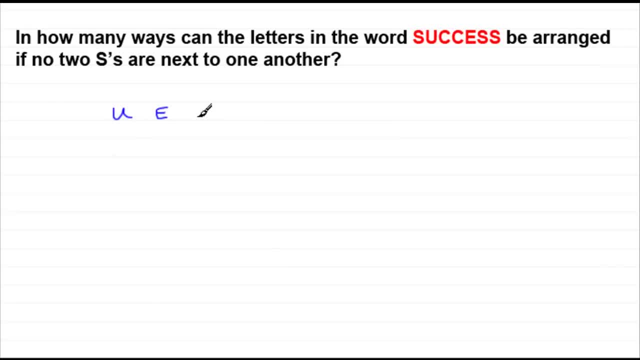 got a U and an E and two C's And I'm going to call those C's C1 and C2 because there's repetition here. And when it comes to the S's, there's three S's I'm going to call 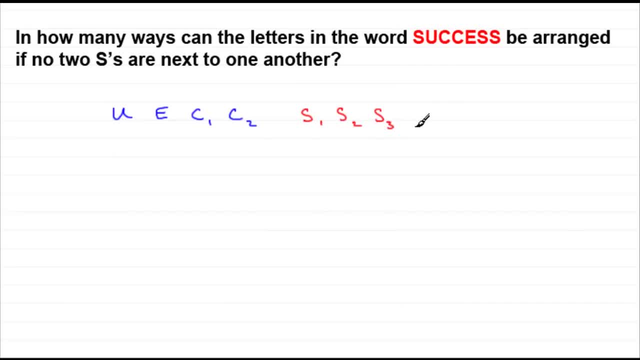 them: S1, S2 and S3.. So we need to think about these letters. here in blue We've got two, four letters, and if we were to leave spaces in between them I would need to have nine dashes. so I put nine dashes down here. let's just say: go one, two. 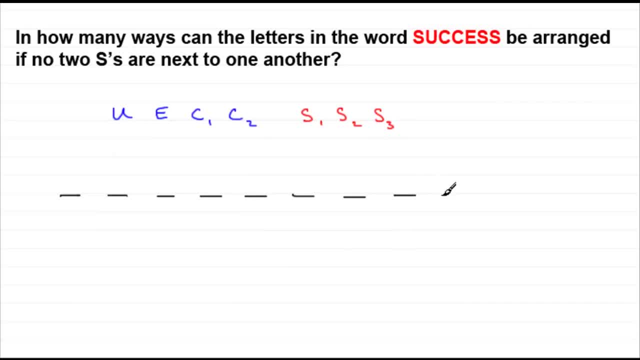 three, four, five, six, seven, eight, nine, and then I would want to insert these letters, so put a, you here say be here, leaving a space between each one: see one and see two. so when it comes to the number of arrangements of the letters that you see, the blue letters, okay, we'll just write that in first arrangements. 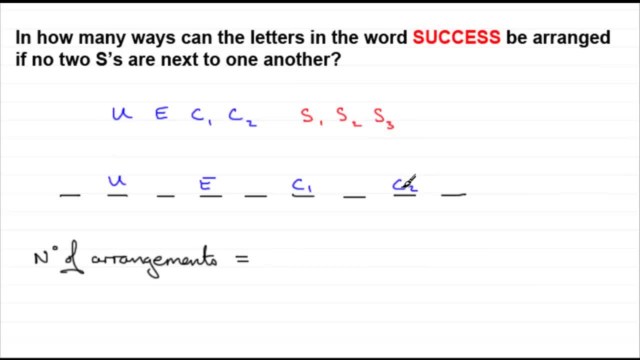 equals. we've got four different letters if we treat the C's as being different, and we know that they can be rearranged amongst themselves for factorial ways. but we've got to be very careful here because we're going to have to be very careful here because we're going to have to. 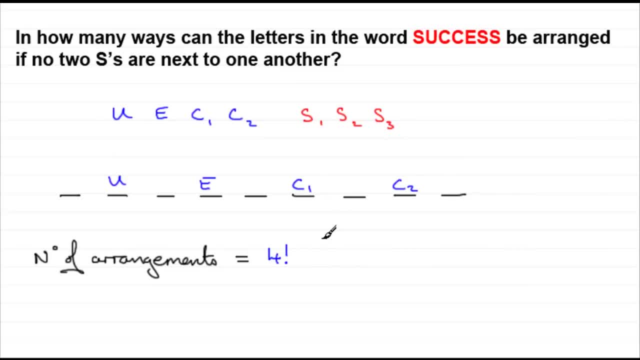 we've got repetition of the C's. so for any one of these four factorial arrangements, the C's, as we discussed earlier when you've got repetition, can be rearranged amongst themselves two factorial ways and we're not going to notice any difference because they won't have subscripts. okay, so we need to. 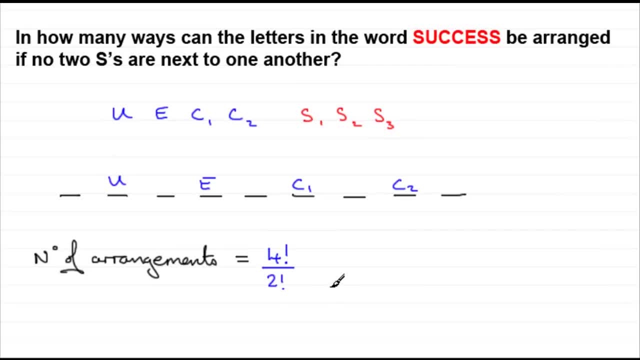 divide this by two: factorial okay. well, that's the number of ways that we can arrange the blue letters. now, when it comes to the S's, we've got to times this by however many ways that we can insert these S's into the spaces. well, for the. 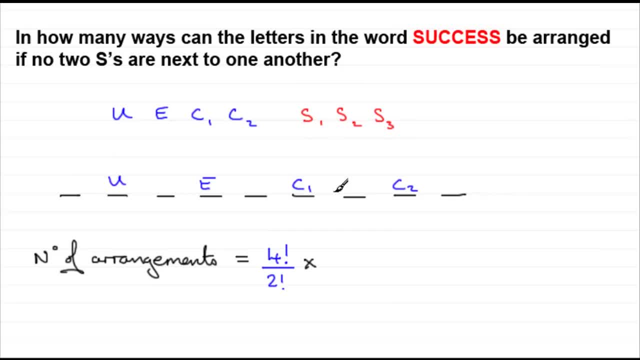 first S, we've got a choice of one, two, three, four, five spaces. so it's got to be times by five. but for any one of the the ways that we place the first S, there's going to only be four spaces left to place the second S. So that's going to be times four. And finally, for the third S, it's going 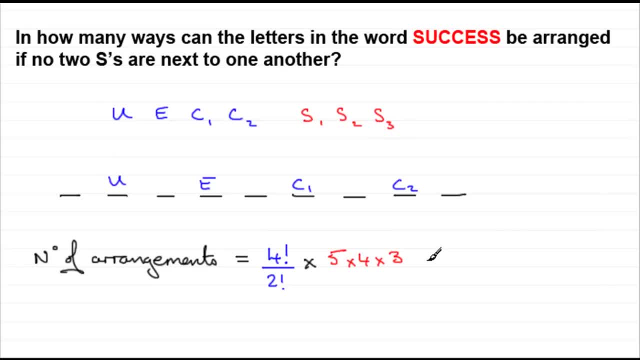 to be got a choice of three possible places. But also with this we've got to be very careful because the S's are different. They're different at the moment because they've got subscripts on. But if you take those subscripts away, any of these arrangements can be rearranged.